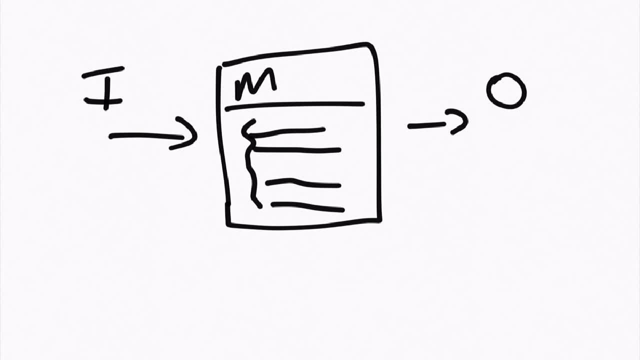 And what do I mean by this? Well, I just want to give in some input and I just want to get out some output. I do not care what goes on in here, And that's abstraction. Abstraction simply means I'm hiding stuff away from the user or the programmer. So if we think about this in terms of 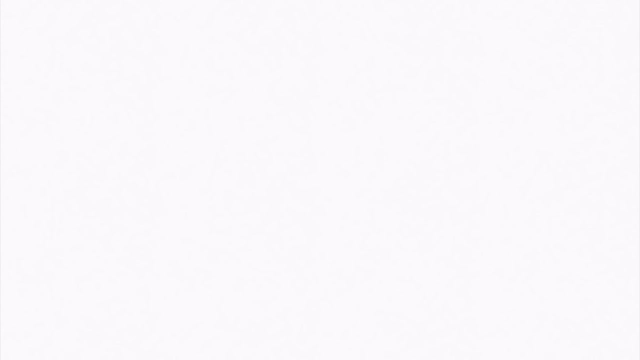 let's say you're in a big software development team and your job is to write the bits. that gets data from the server, And then it's someone else's job to show the data on a screen. So they're going to communicate with you and say please go get this. And you'll say: 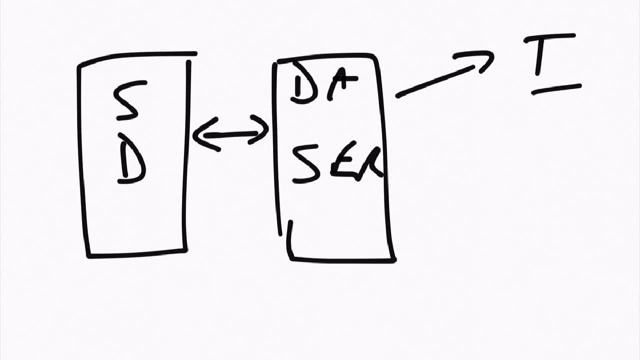 no problem, I'll go get it And off you go to the big bad world of the internet, which returns you the data. Now the guy writing this display code doesn't really care how you get the data. He just wants to say to you: get me some data And then it's up to you to get that data. 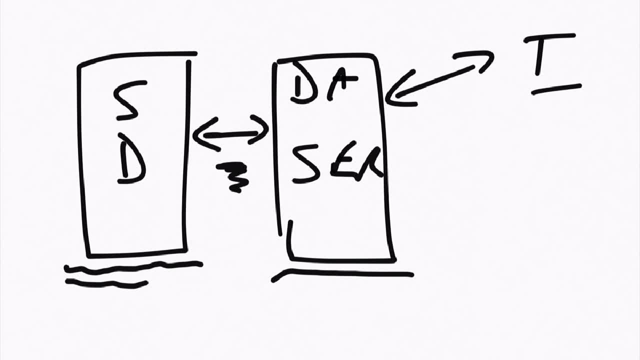 however you do it, It doesn't matter. That's the whole point. This software guy doesn't need to know how you get it. You just simply go and get it from the internet, And then you, of course, return it to the display guy. And that's what abstraction is It's hiding away. 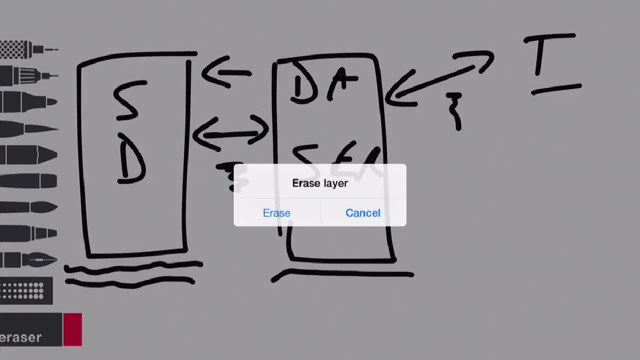 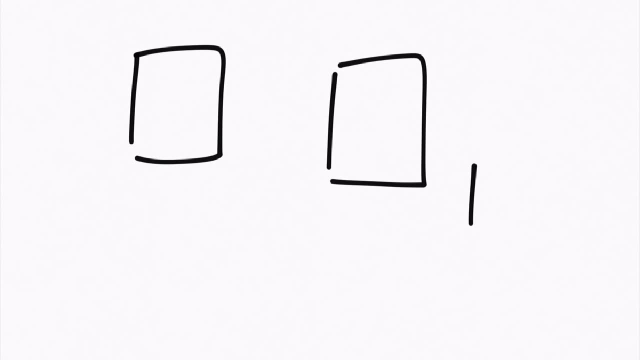 functionality, And when you do that, you get this beautiful effect in programming, which is everything starts to become kind of modular. So, again, like Lego blocks, we have, say, the view, we have the database, we have the internet and we have some other guy on. 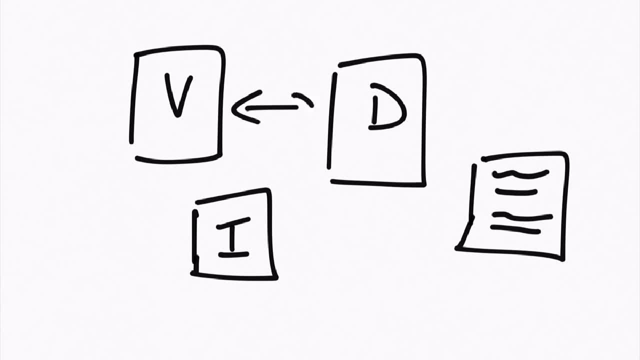 your team. that doesn't do very much. And then you get this beautiful effect in programming, which is pretty much, And they can all kind of talk to each other because they know how to talk in terms of input and output. So, as long as your thing, your bit of code, accepts a certain input and puts out.